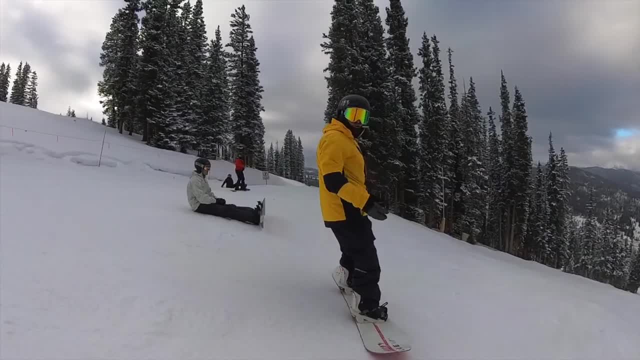 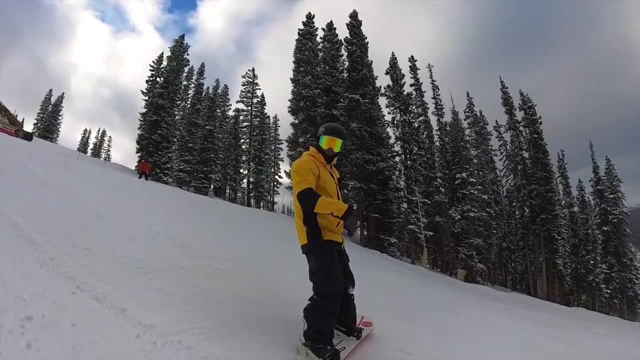 So we're going down this slope. I'm going to be going 90 and I can control my speed by how low my toes go or how high. You don't want to put your toes too low or you're going to flip over. Also, I can then go from 90 degrees to like 60. I'm going to pick up the speed, go back to 90 and I can. 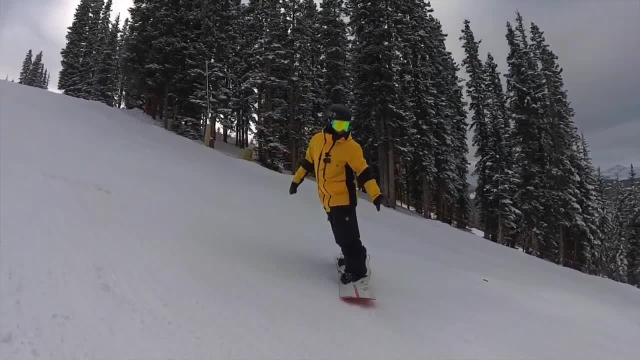 slow down. I can do the same thing on my toe side edge so I can control my speed. being 90 degrees on my toe side edge, I can go 60 degrees. I'm going to go a lot faster, go back to 90. It's a very 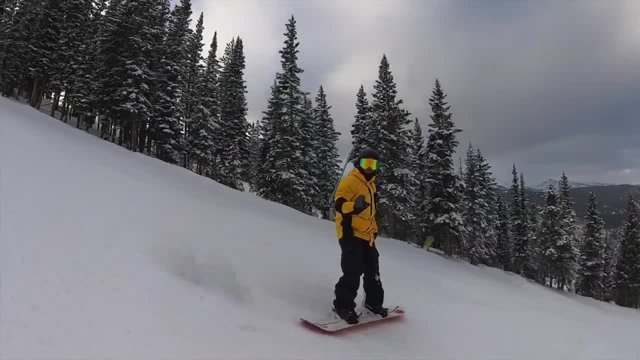 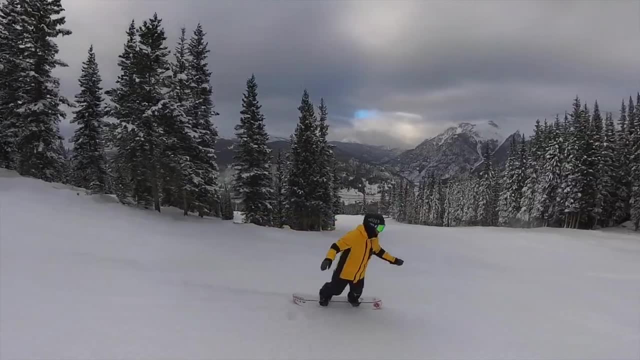 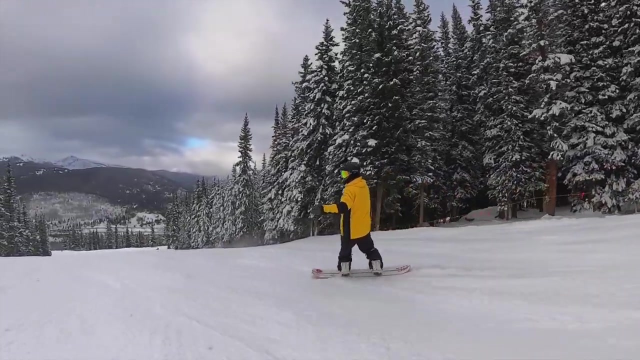 basic way to control your speed on the mountain. The other way, once you get a little past beginner, is by traversing across the run. So if I want to not go too fast, I'll go all the way across the run managing my speed. Come back around and I'm not going to be going super duper fast across the run. 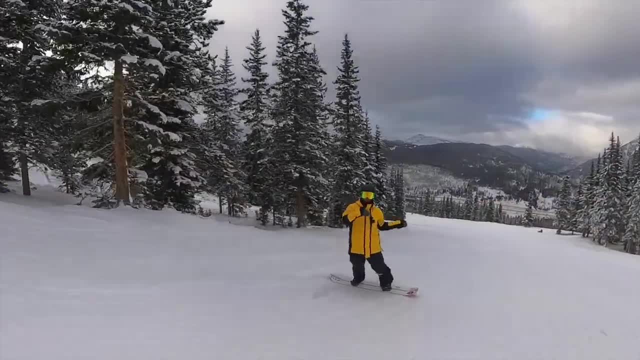 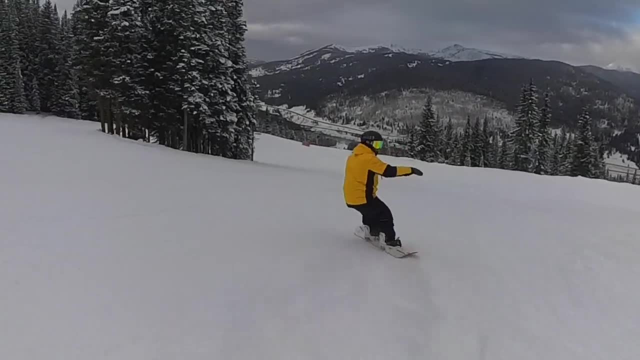 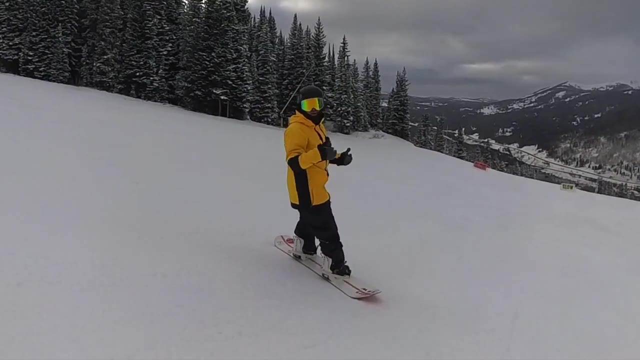 as opposed to straight down. If we go straight down the run, we're going to go really fast Here. I'll show you: We don't want to snowboard like that. It's dangerous. There might be moments where we need to do that, but overall that's not how we want to snowboard. Now, if this is already making 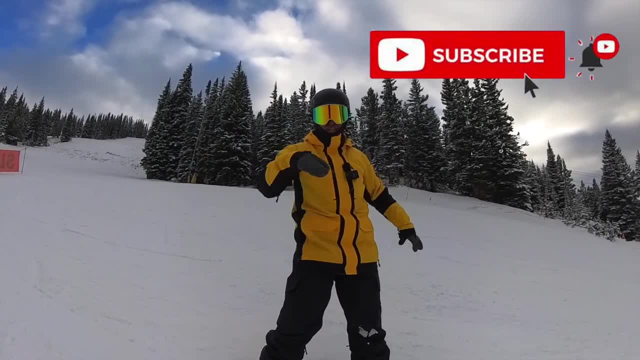 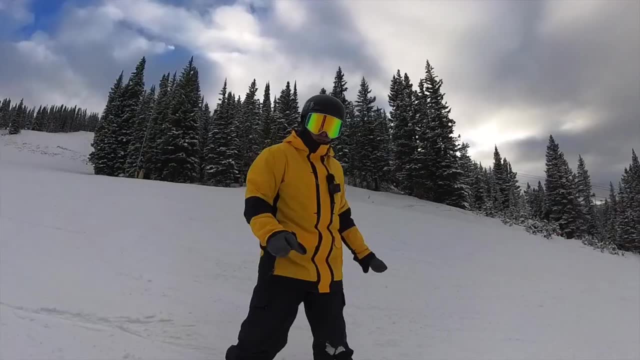 sense, make sure you subscribe to my channel. I cover all kinds of snowboard skills and everything, but also we just do like daily vlogs, just experience on the mountain. It's a really fun channel. You want to subscribe, Trust me. you want to hit that button, Okay. so now let's go to the 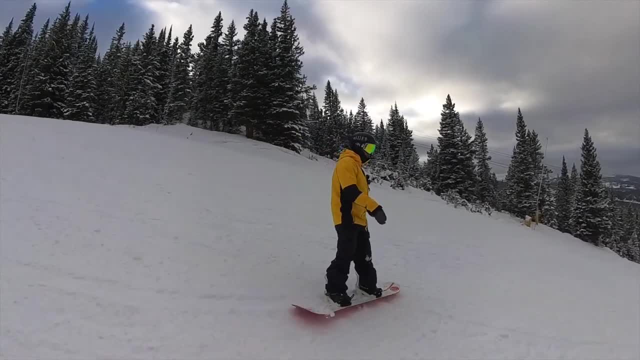 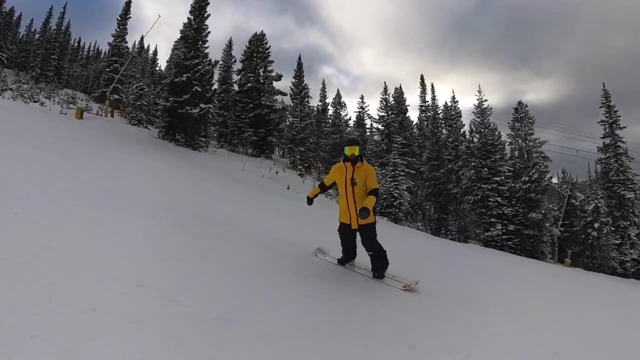 intermediate level. Let's say we can s-turn So we can come down the mountain. You know we can turn. Now, the way we can lose speed is by doing what we call a counter rotation. This is a counter rotation: We're keeping our body and our eyes. 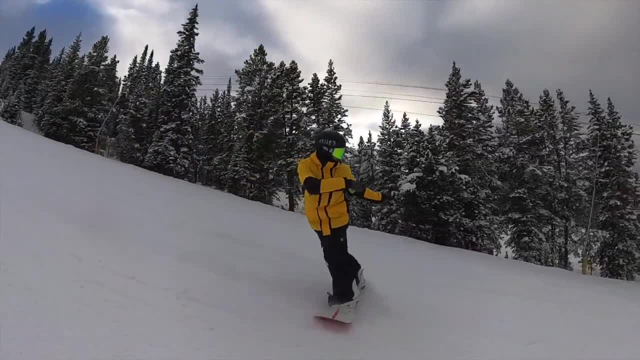 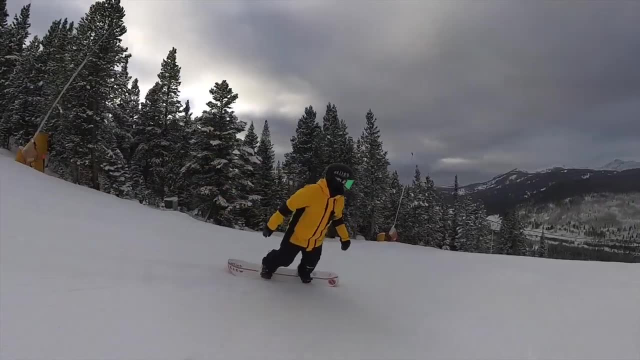 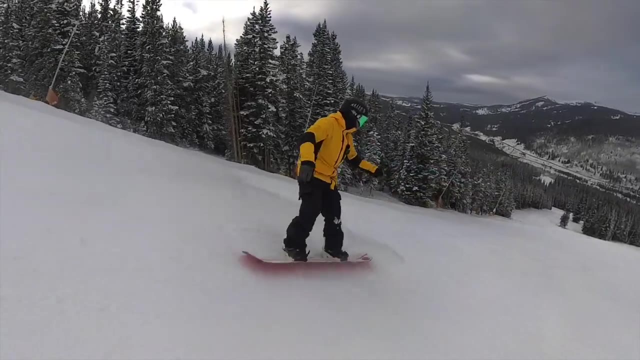 everything going down the run and in a turn we can counter rotate and come back. Now we can do this on our heel side edge too, So we can be toes heels back, Heels back, Counter rotating, Just shaving off that speed. Once again, anytime our board goes 90 degrees we're slowing down. 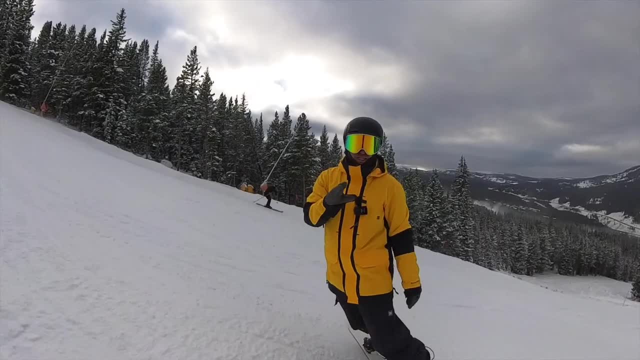 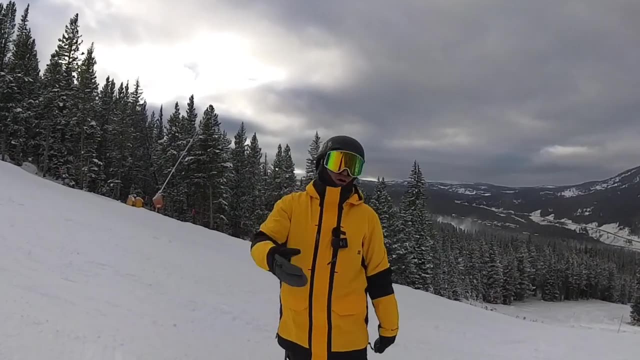 Anytime our board's not 90, we're speeding up And if you're into speed, you want to snowboard fast or you want to control your speed, consider snagging evolution sticker. Supports the dream. It's how we do this for a living. Also, I hear it helps your speed control on the mountain. You know what I'm? 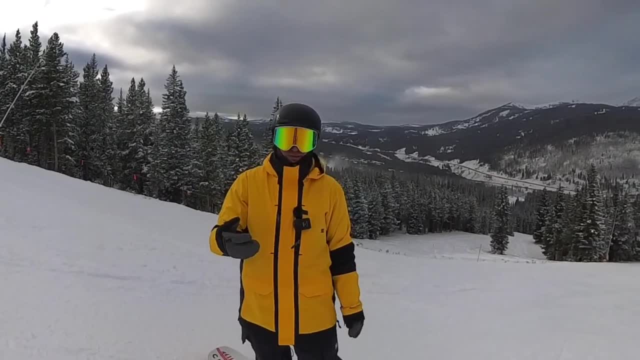 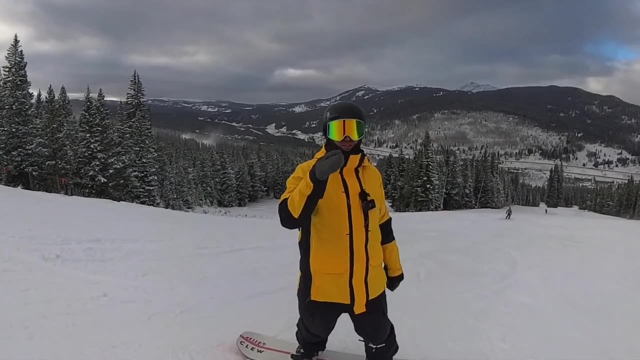 saying We're going to kind of step now into the expert level, which is that counter rotation Kind of like more ramped up, And I'm going to do the best job explaining this, but I feel like I've never done this before. So I'm going to hit expert level and it all becomes fluid, And that's when 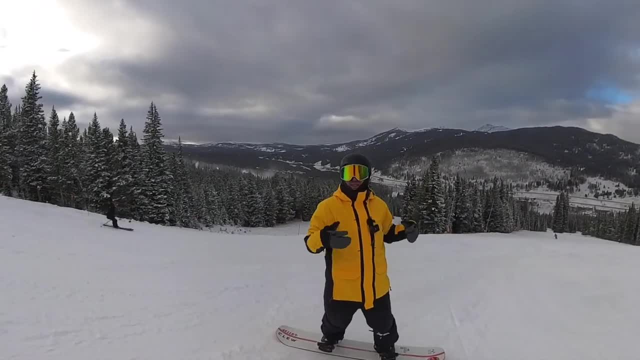 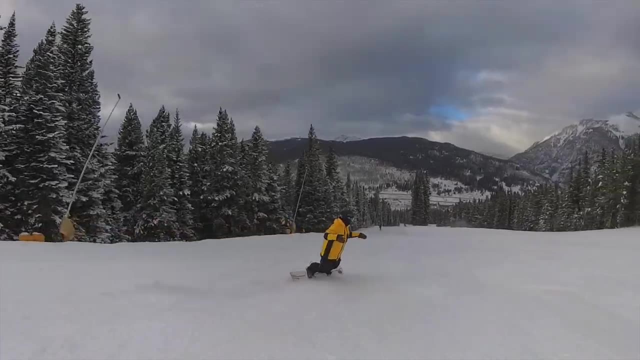 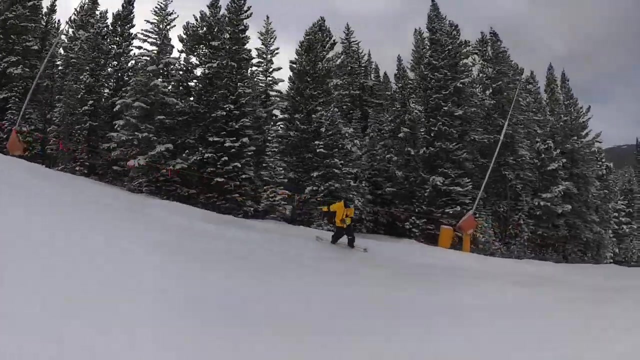 you hit. expert level is when you use every form of slowing down in ripping. Okay, here we go. So let's get some speed. So I'm going to go edge to edge. I'm going to go cross run- slow down a little bit. Cross run a little slow, I'm still a little fast. Spray, Just like little kick spray, right, 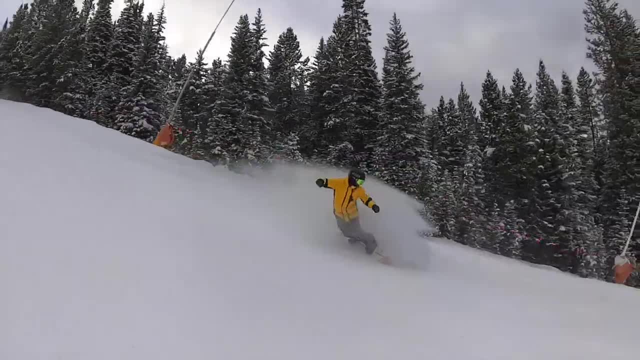 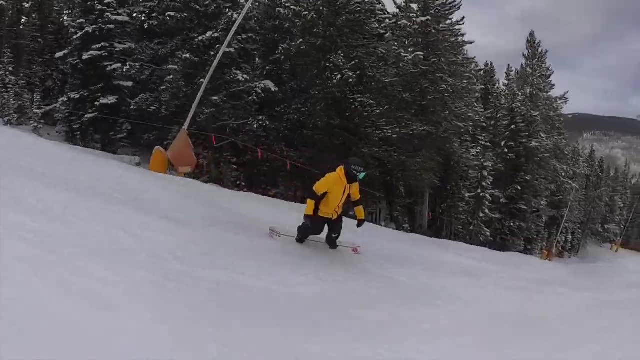 here, Not full 90.. It's cool because it throws up a cloud, But it also slows me down. Go full 90 a little bit, You know. I mean just go 90, slow down, Then pick it back up. Spray here. 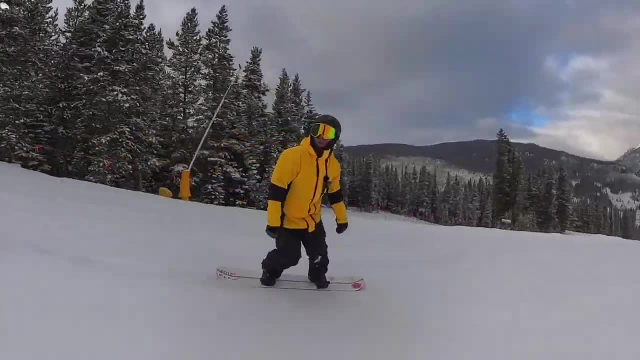 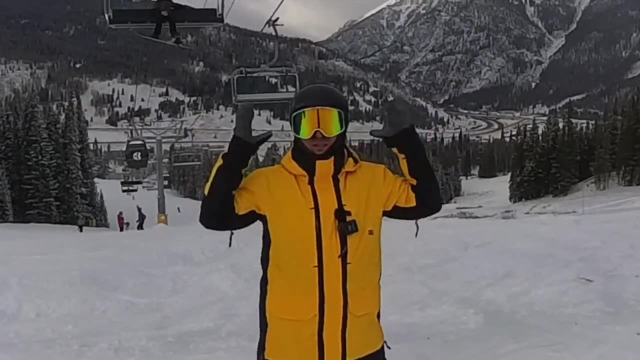 All of this is speed management. So it hit me when I was doing that and like fully opened it up. But expert speed management is when you take literally everything I showed you in the beginning, The beginner speed management to the intermediate speed management. You take all of that and you 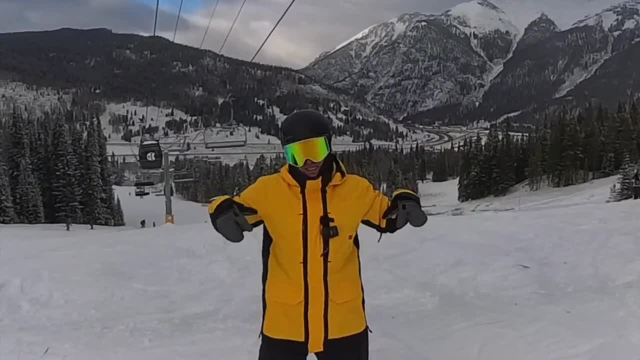 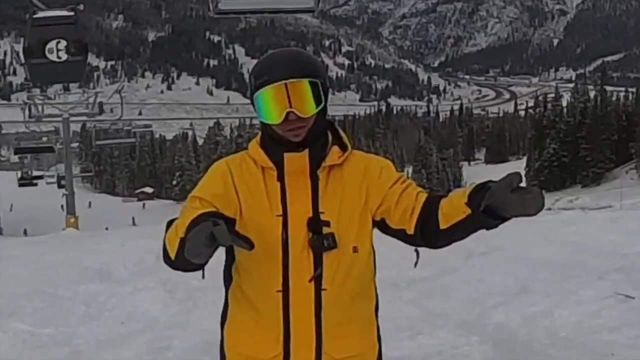 put it into one, And that's how you become an expert at managing your speed. When, at any moment or scenario, you need to, you know how to do the speed management that's necessary to not be cruising. Also, the spraying of the snow- That's a great way to to shut off some speed. I totally 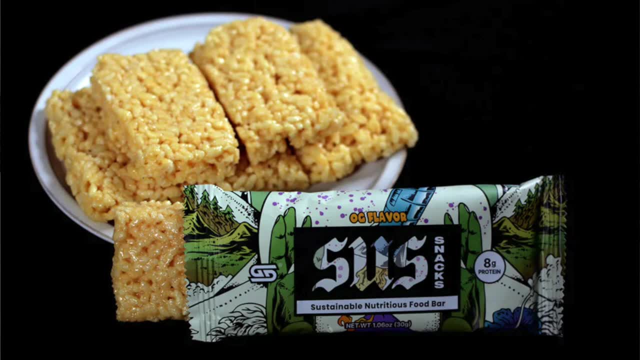 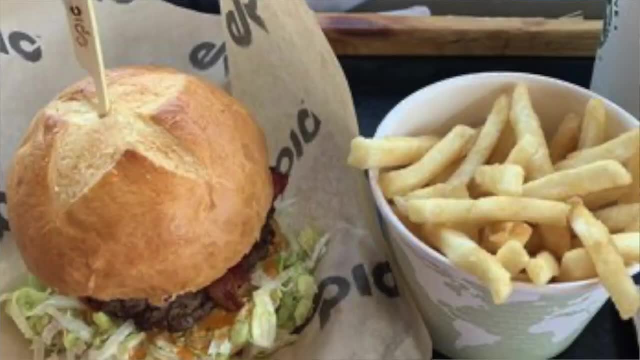 almost forgot. We gotta mention the video sponsor, Gamersup. They just released these energy bars, So it's a water infused energy drink. Now they got energy bars and yo, we're out here snowboarding, We're out here ripping all the time. Most of the time you go in the lodge and buy expensive food. 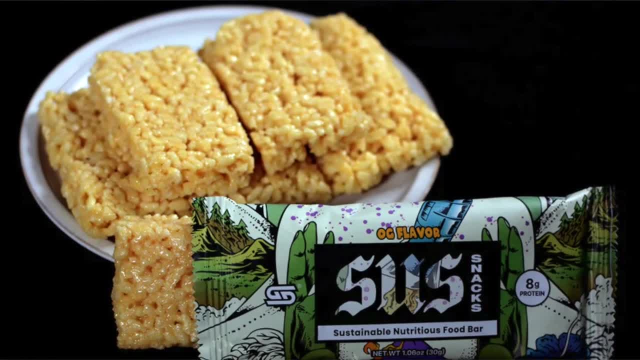 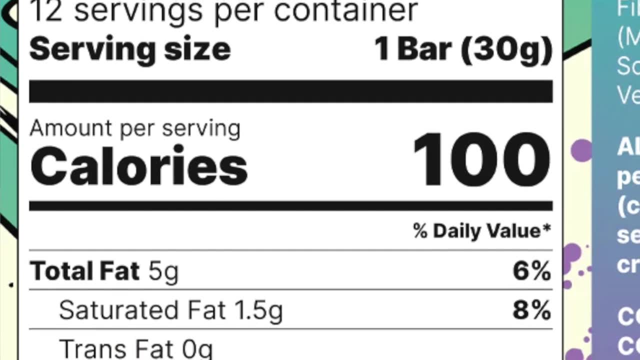 because you think you're really hungry, but you're really not that hungry And an energy bar is all you need to be good on the mountain. And this is a Rice Krispie energy bar. I absolutely love Rice Krispies. Now I've got an energy bar. It's only 100 calories, One gram of sugar, No added sugar. 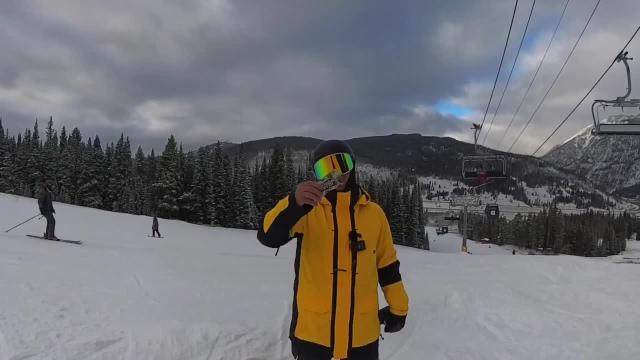 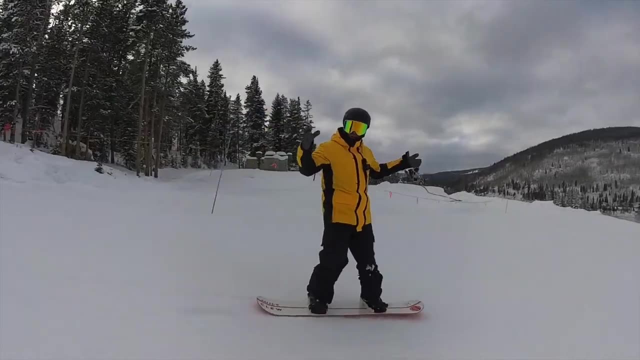 This stuff tastes incredible. It's good for you. Gamersup Link: in the description. Use my code, buck 10.. Save 10% off. And also you can get the water infused energy drink. Let's get in this last section. Let's rip it All right, guys, we're gonna put all of the skills and drills. Just learn and